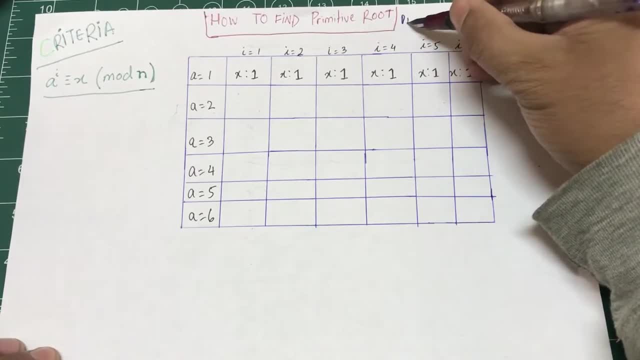 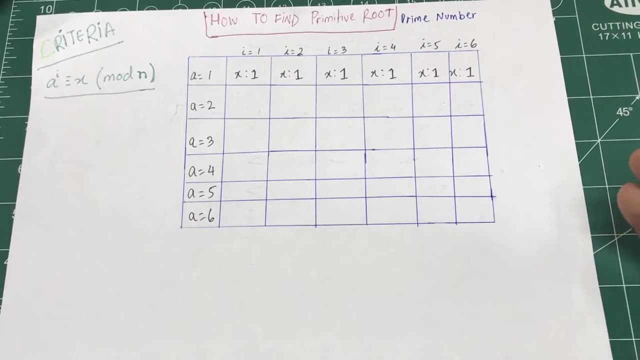 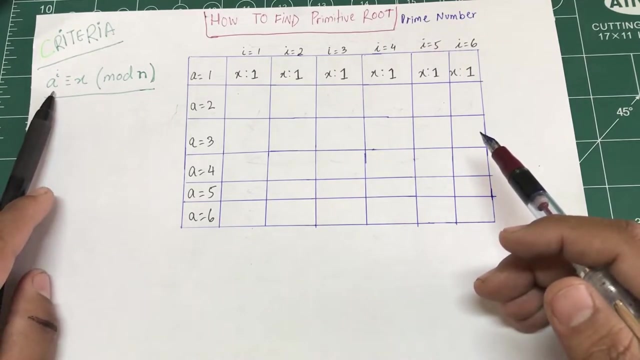 to actually find primitive root of a prime number. okay, I don't know. I mean, this is how I learned it and I like this. I mean, the way I found this way is to the easiest way to actually find that. so the criteria for finding a primitive root is actually this, a number that 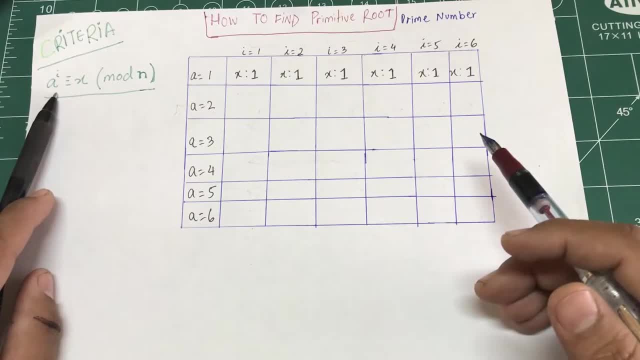 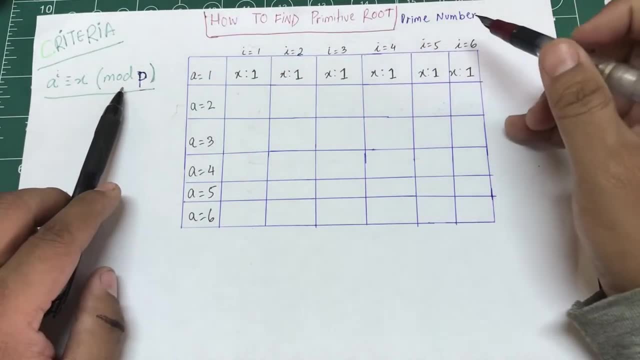 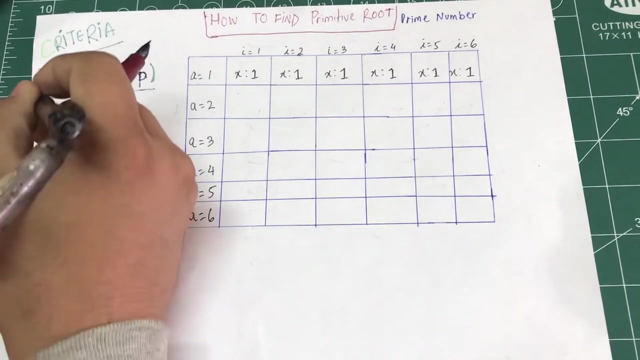 you're trying to find. so let's say you have a number like this and let's, instead of n, let's just make this P. so we're trying to find a primitive root of a prime number. so the criteria that I need to have is just. first thing I need to do is actually to solve for to find Euler's quotient. 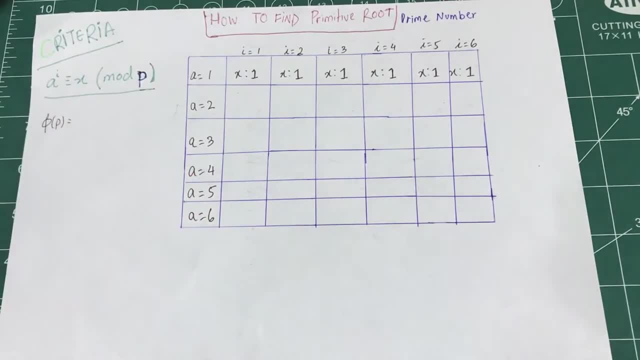 function of that prime number. alright, so Euler's quotient function actually gives me the range of of what numbers that I want to try. I mean, you will see as we, as we do an example. so so let's say k, i want to find if i have a prime is equals. 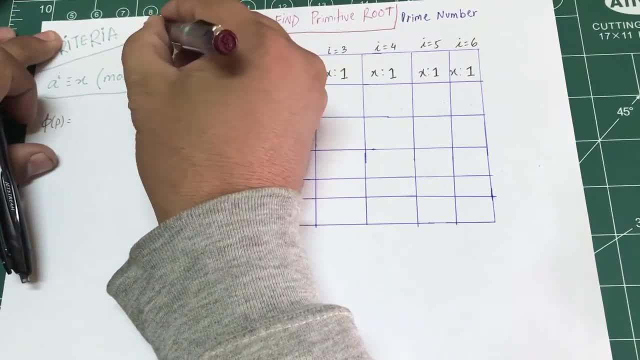 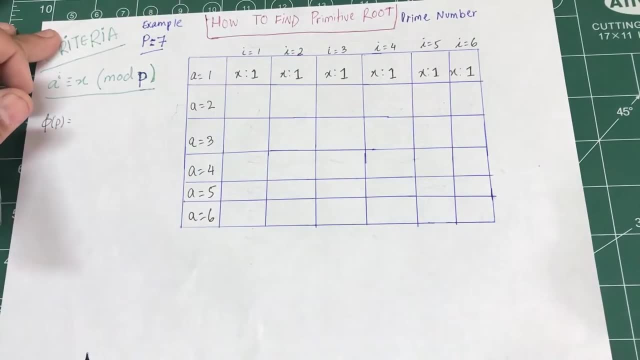 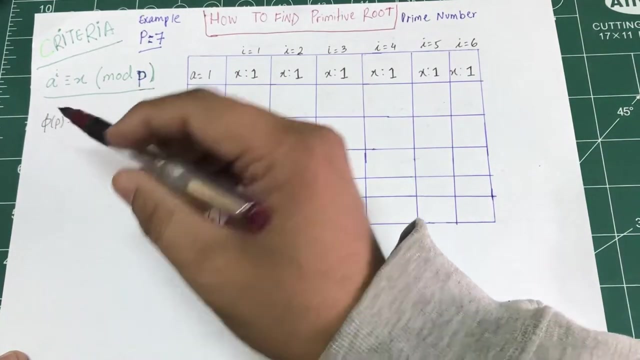 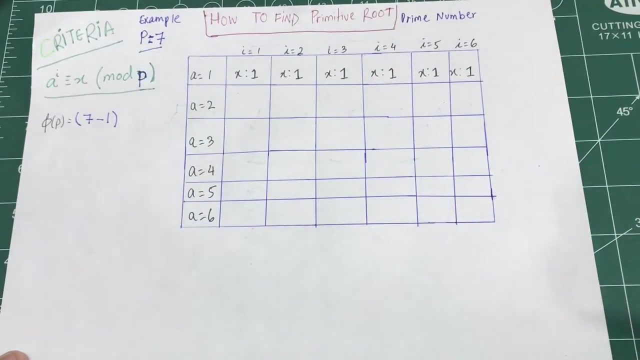 to 7. so in our example- so here's our example- our prime is equals to 7 and we want to find primitive roots of 7. so the criteria is so: the euler torsion function for prime number is actually 7 minus 1. if you remember it from from rsa, euler torsion function is for rsa was. 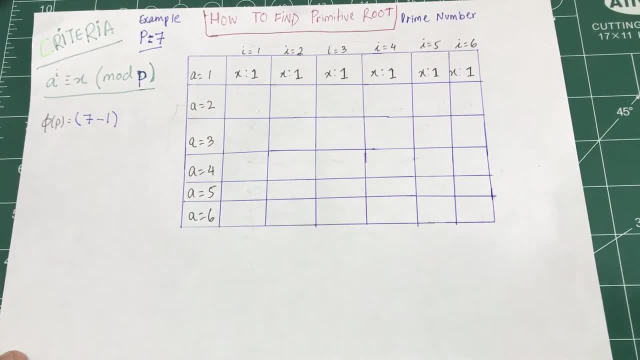 because we have to choose two prime numbers. one is p and one is q. so euler torsion function is basically prime minus 1, the second prime minus 1 and you just multiply them to get euler torsion function. here the euler torsion function is actually just going to give me a range range. 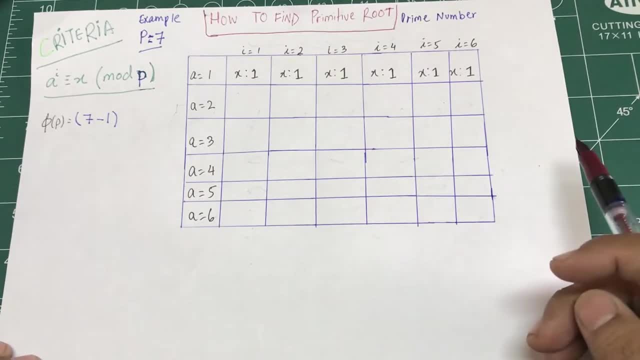 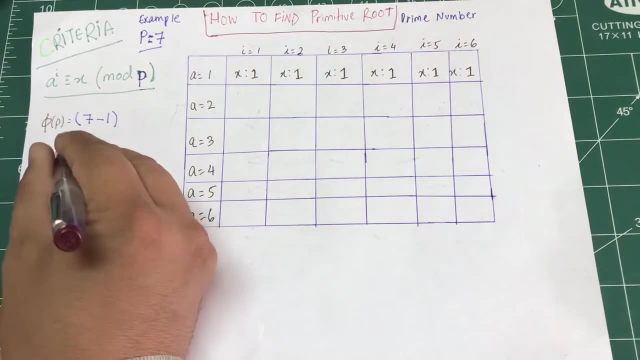 of numbers. so let's say, in our example we want to find primitive root of 7, so the euler torsion function for this is going to be the prime minus 1, so this is going to be 6, all right. so that's why i have 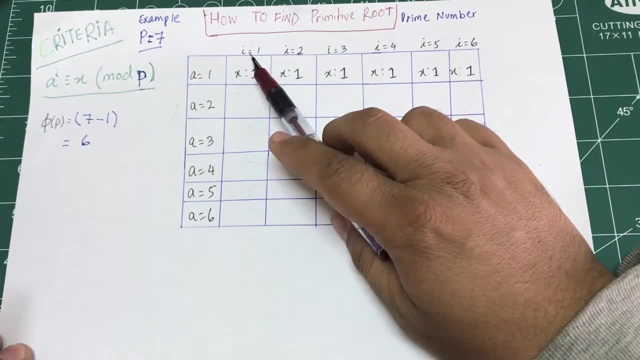 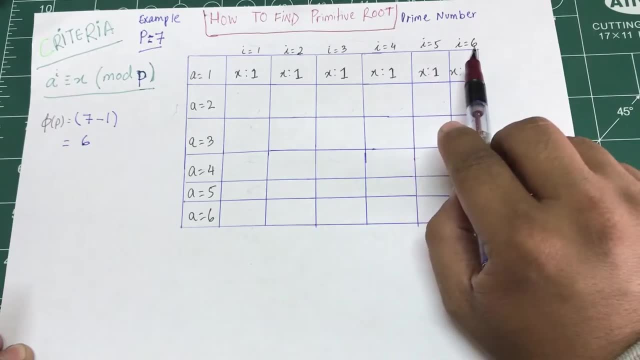 6 entries. if you can see over here i have: i is equals to 1, i is equals to 2, i is equals to 3, i is equals to 4, i is equals to 5, i is equals to 6. all right, so what we do to find primitive? 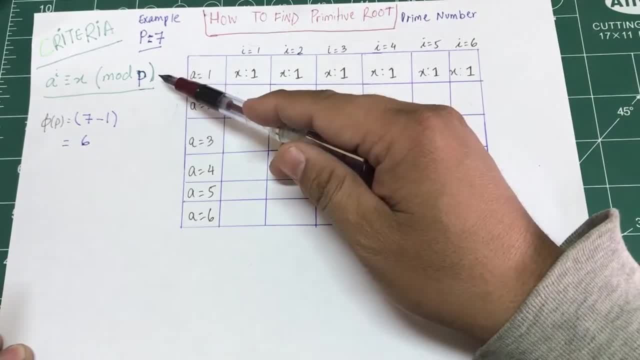 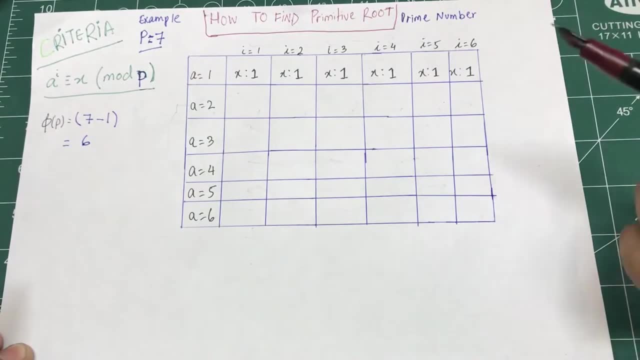 roots. we are actually continuously checking this criteria. if this criteria meets, okay, and the reason we find primitive roots. primitive roots are those specific number that generates and this entire sequence up till 6, all right. primitive roots are those number which generates the entire sequence up till this number, up till this euler torsion function. 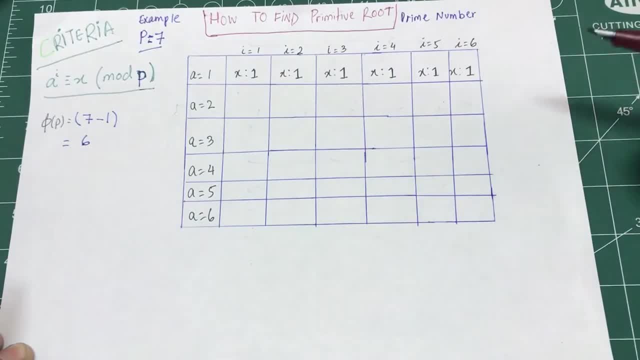 let's say if you have a prime, let's say 23, 23 is a prime number. so the euler torsion function of 23 is going to be 23 minus 122. so let's try to find out a number. primitive root is a number that generates this entire sequence. 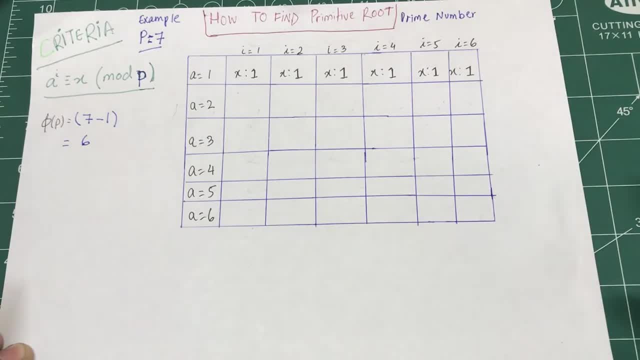 up till 22. i don't care about in which order is coming in, i just only care about: will this number generate this entire sequence, this entire number sequence from 1 to 22, whichever order it is. so so the checking criteria for this is: we're just checking. 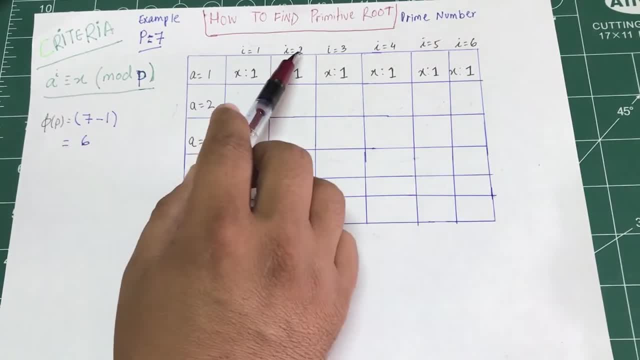 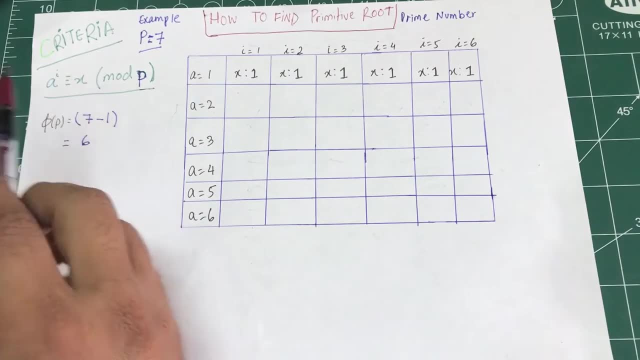 single number. in place of i, we're going to use one, two, three, four, five, six, because that's what my euler torsion function is, and a is also going to be one, two, three, four, five, six, seven, eight, nine, ten, uh sorry, a is equals to be a from all the way up to one, two, six. why? because our prime number is 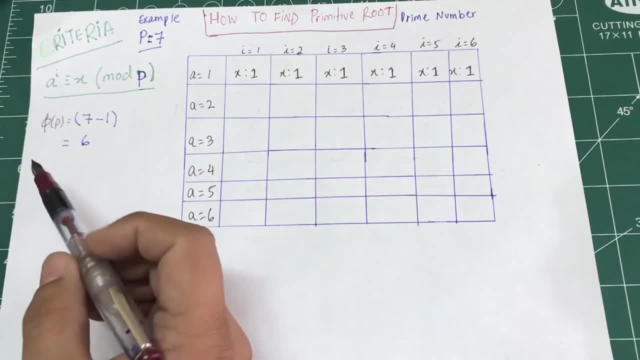 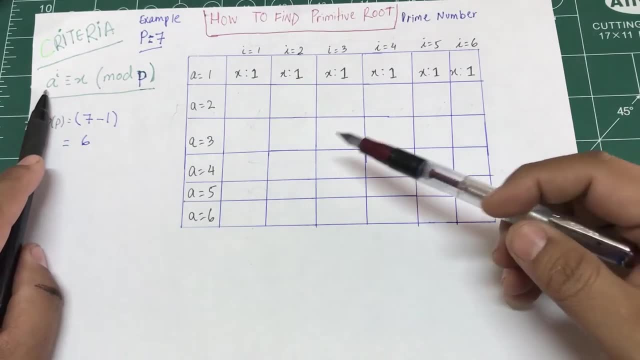 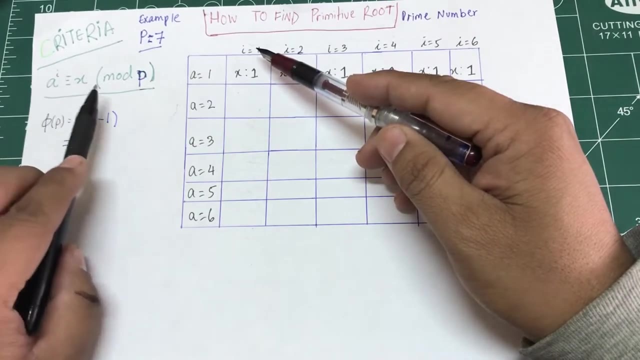 seven. so let's do this. i already saw one for you, because one is quite easy. so here's what we're doing. we're doing this in place of a, let's take one, and in place of i, let's take one. one raised to one is one. you take mod with seven. what do you get? one, because when you have a number, 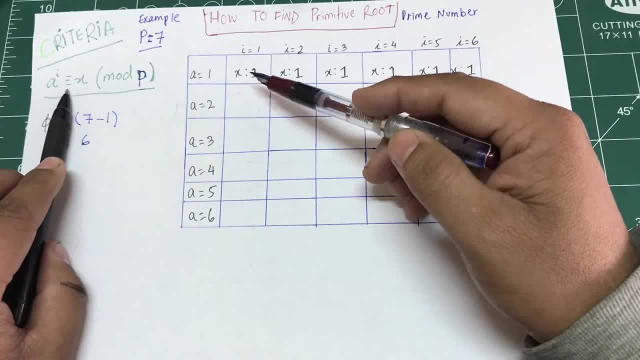 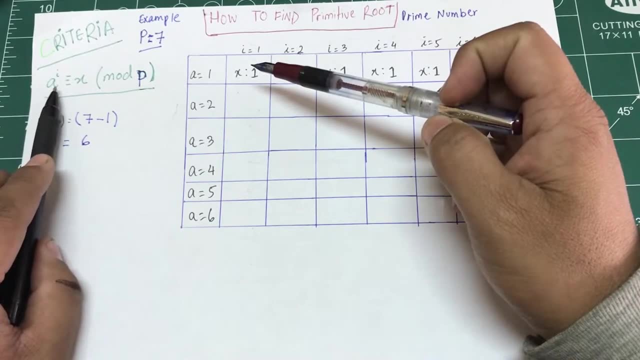 that is smaller, and observe this congruence operator, which is there. this congruence operator is there because there is going to be many of these values, many of these values which is going to map the the to this particular value. remember, in congruence operator, when we did. 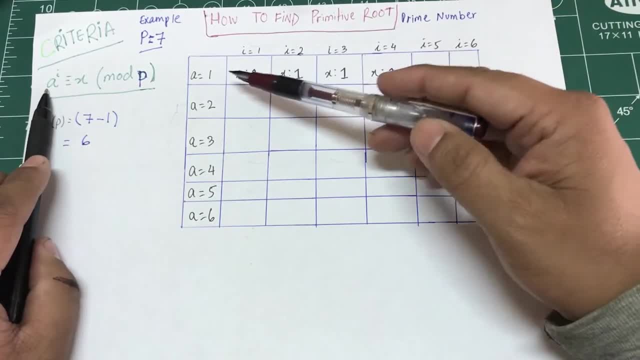 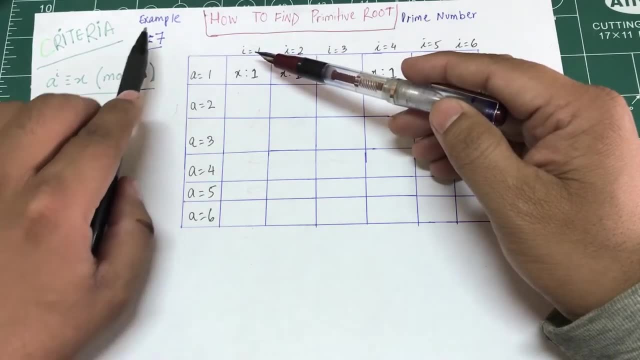 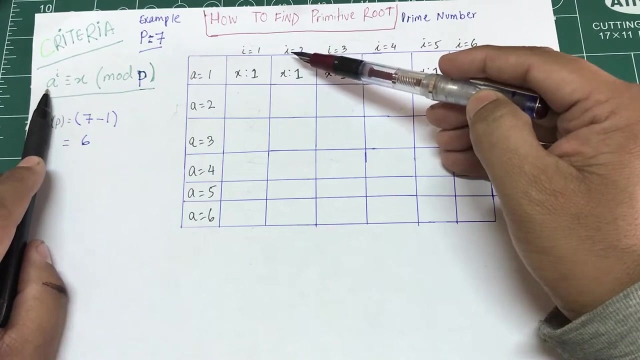 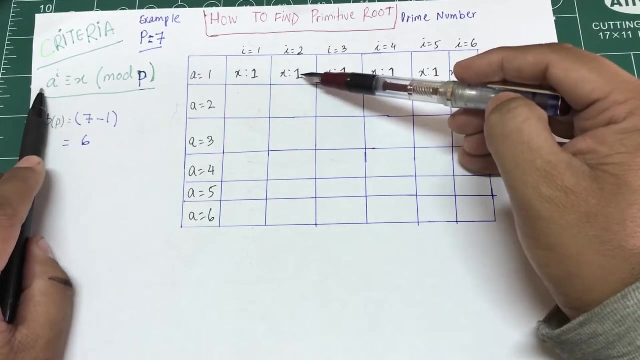 modulo arithmetic. so let's do this. so in place of a, we'll take one, in place of i, we will take one. so one raised to one is one. mod seven would give me one. all right. one raised to two. one raised to two would give me one. one. mod seven is one. one raised to three. 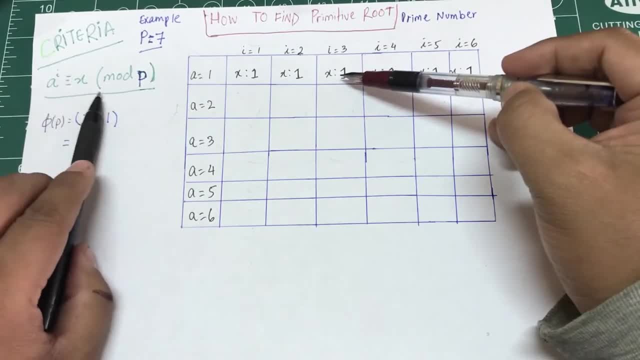 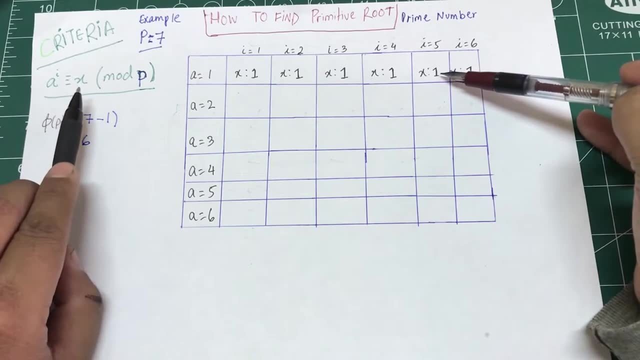 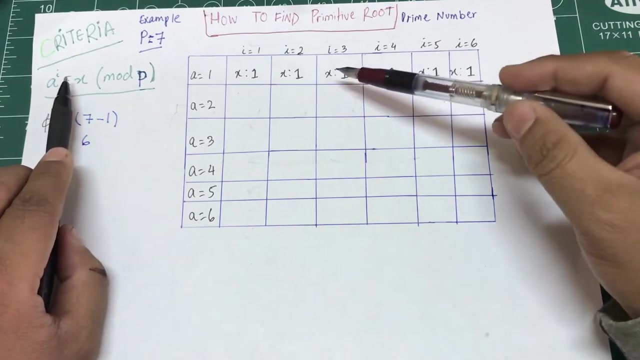 mod seven would give me one. one raised to four: mode seven give me one. one raised to five mods: one raised to five- mod seven would give me one. one raised to six- mod seven would give me one. all right, so this is how you're going to generate this. okay, so let's do number two. 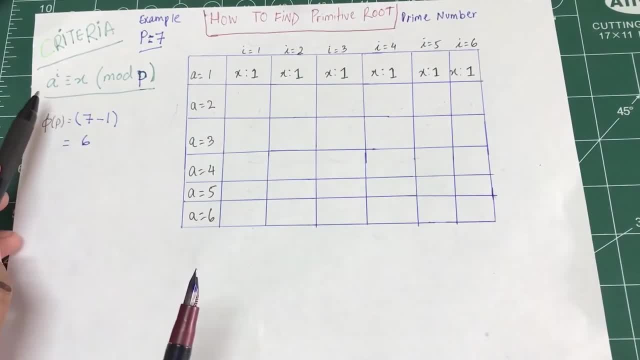 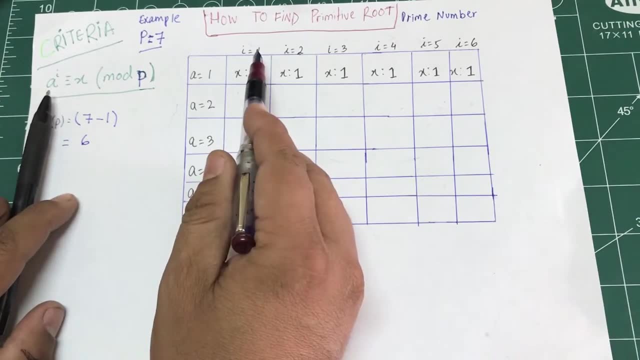 so. so now what we're going to do is this: let's say two. let's take in place of no, mod nine. so we're going to write this as mmc times: x minus x. let's say 케 place of a. let's take two. two raised to one. two raised to one, mod seven. two raised to one is what? 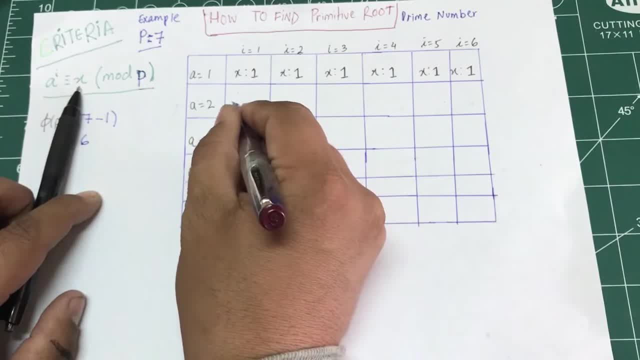 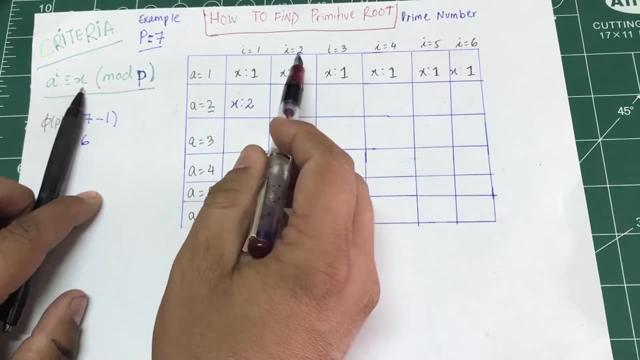 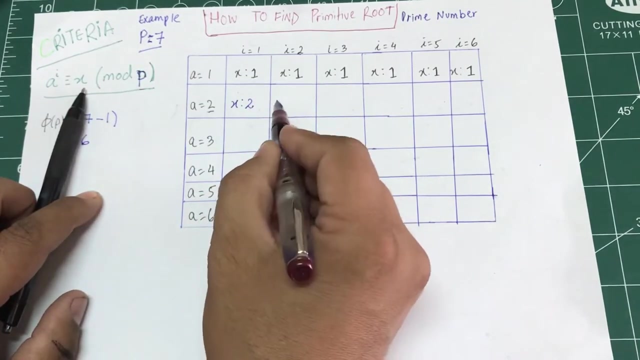 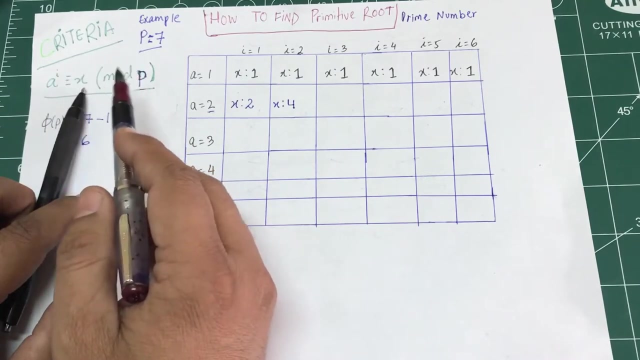 two mod seven would give me two, all right. so let's do this two. two raised to two, mod seven. two raised to two is four mod seven would give me four, all right. two raised to three is eight mod seven. that would give me two raised to one. 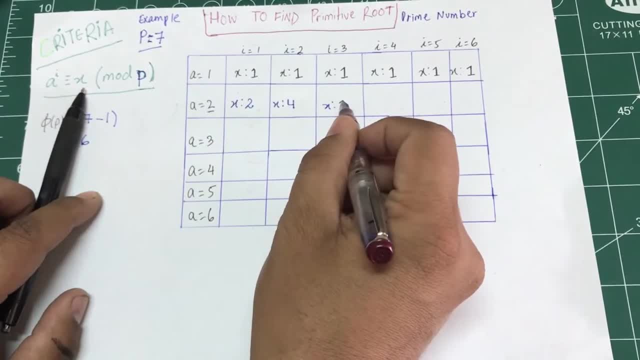 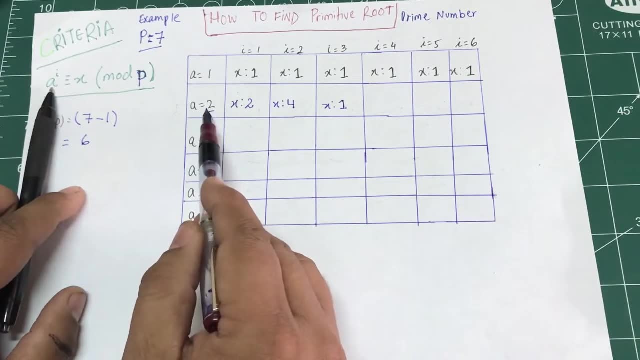 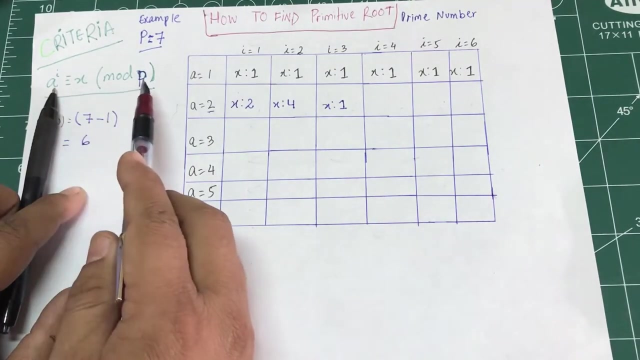 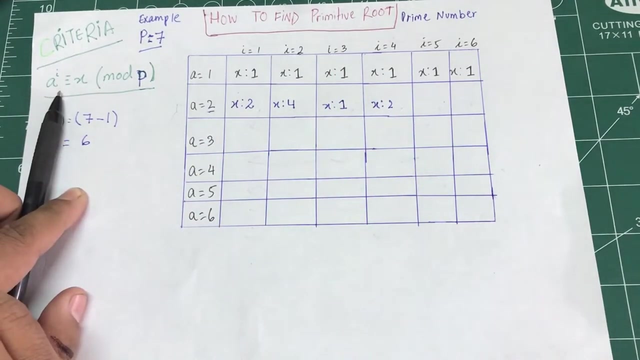 all right, let's try two raised to four. two raised to four is sixteen. so in place of a, we're using two, in place of five we're using four. so two raised to four is sixteen. sixteen mod seven would give me what two. two raised to five is 32, 32 mod seven would give me. 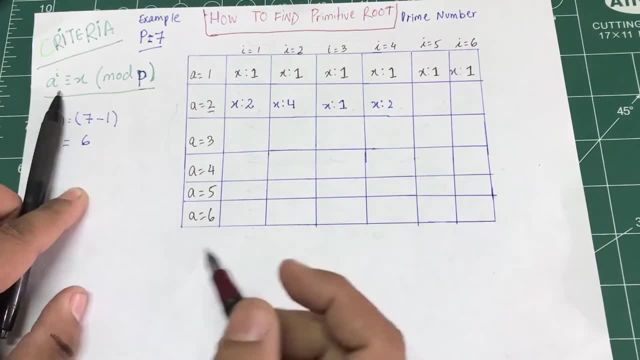 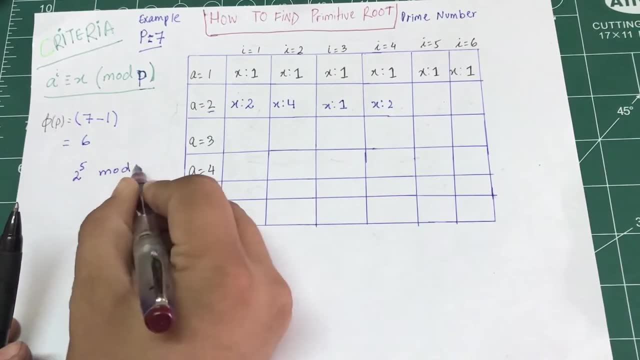 four, 32 mod seven, would give me, if you, if you forgot how we're doing it. so let's say two raised to five mod seven. two raised to five is 32 mod seven. so seven divided by 32, seven times four, is 28 and I'm getting a remainder of four. hence we have X is. 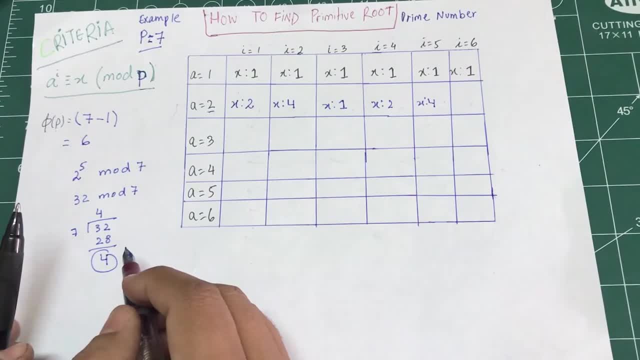 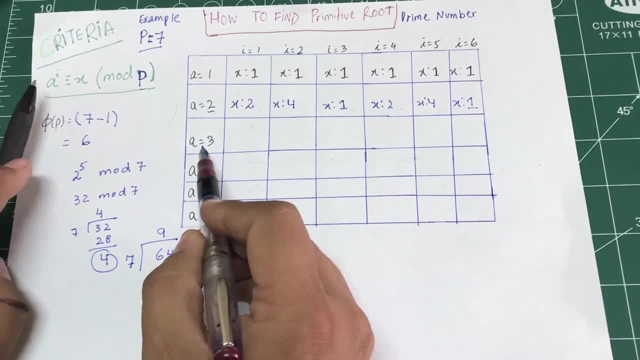 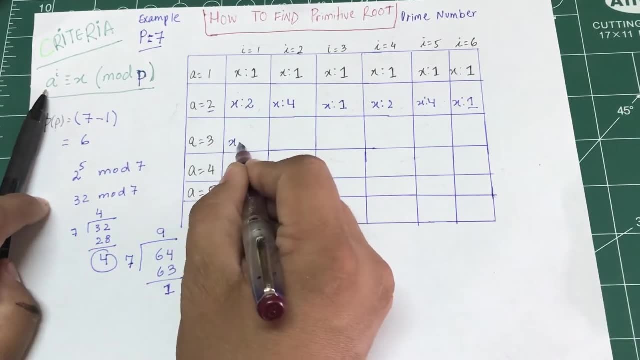 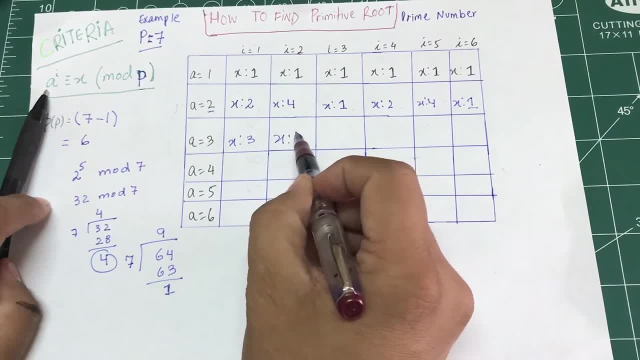 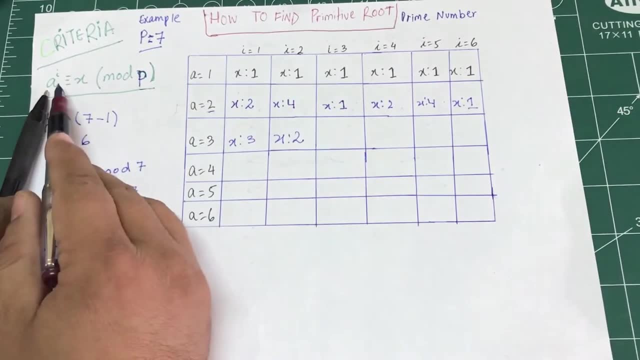 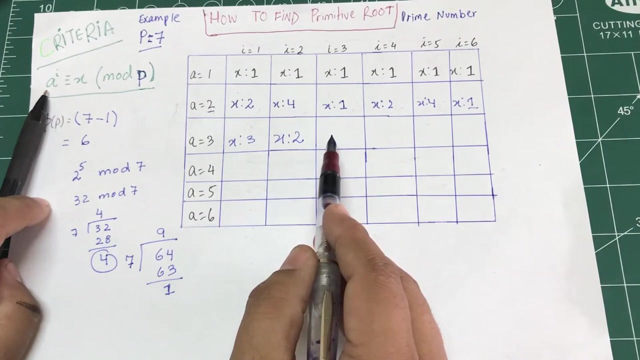 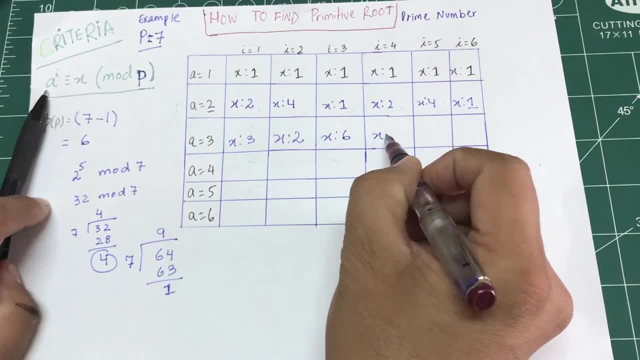 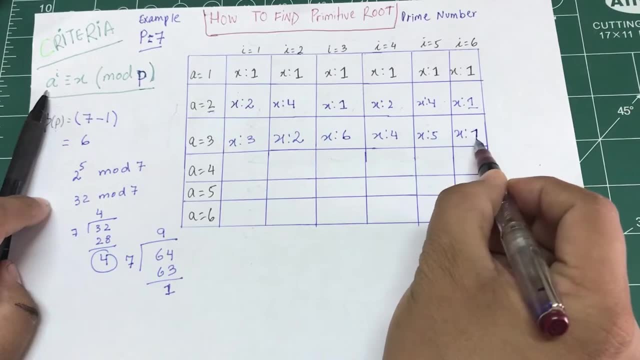 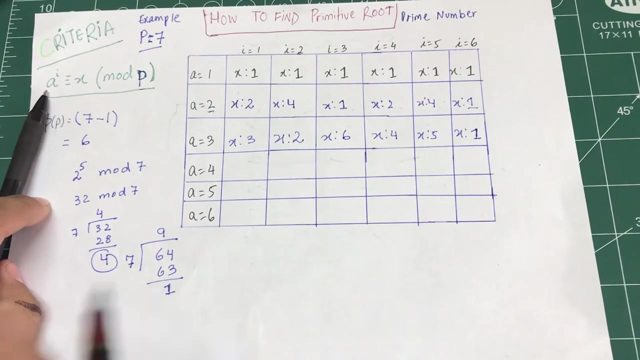 we're just taking the remainder and so on. so let me just quickly populate this. i hope you're getting an idea. what is it that i'm trying to do here? so let me quickly, uh, populate this, uh, so, uh, so you then, then i'll tell you which one is primitive. 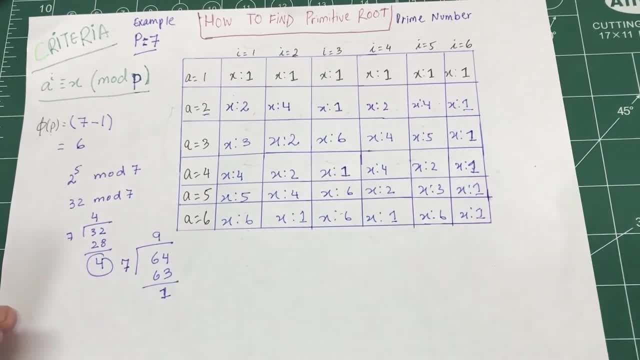 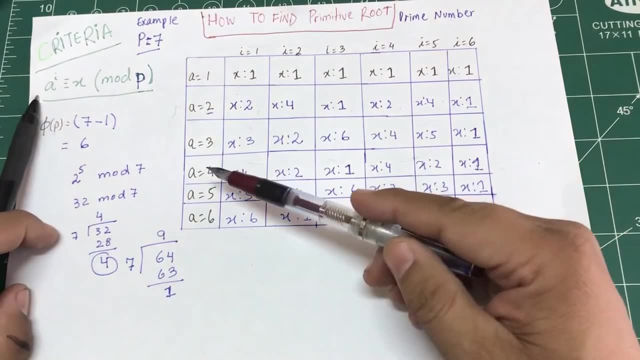 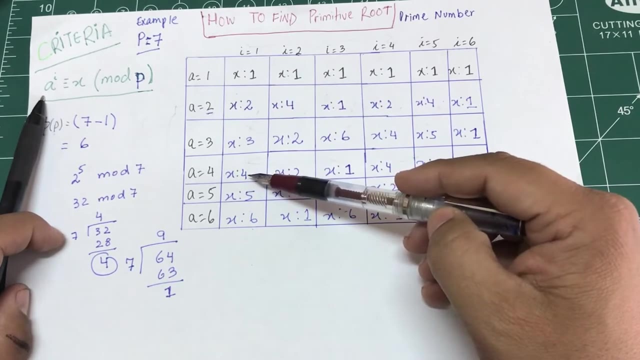 root, okay, so i just actually populated this and, uh, just to show you, okay, let's recap how we're calculating this, how we are fulfilling this criteria: taking a- whatever that number is, which is 4, and raising it to individual power. so 4 raised to 1 mod 7 would give me 4. 4 raised to 2. 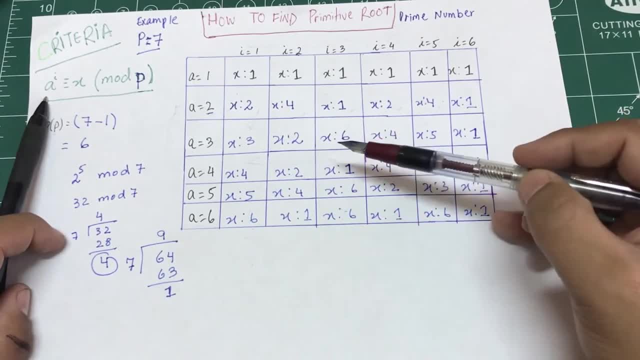 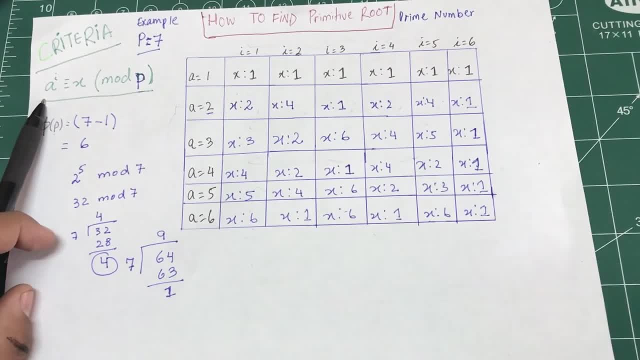 definition of primitive root is a number. primitive root is the number that generates an entire sequence up till p minus 1. okay, so the definition of primitive root is a particular number which is a generator that actually generates an entire number sequence in different order, up till p minus 1, which is that euler tuition criteria. 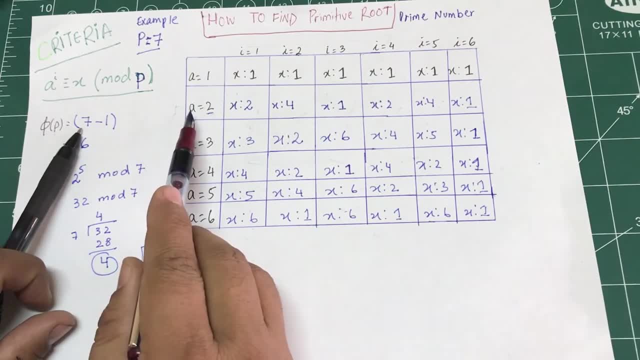 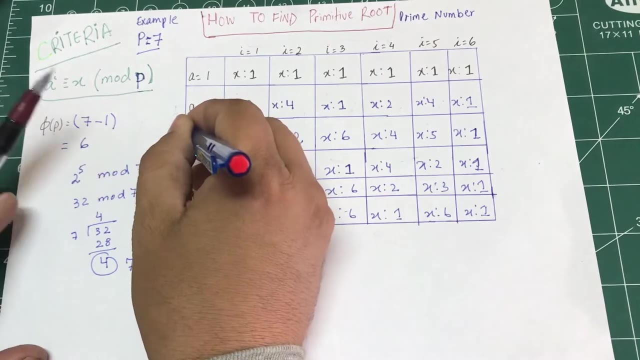 so if you were to observe this, what, what value of a is actually generating an entire sequence of that number without repeating itself within that domain of p minus 1? so if you were to look at it, there's only there are two numbers which are doing this. 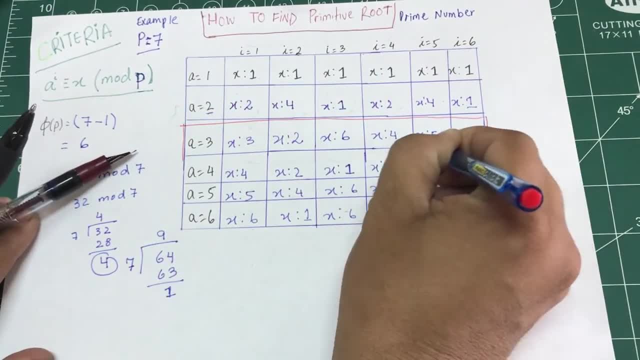 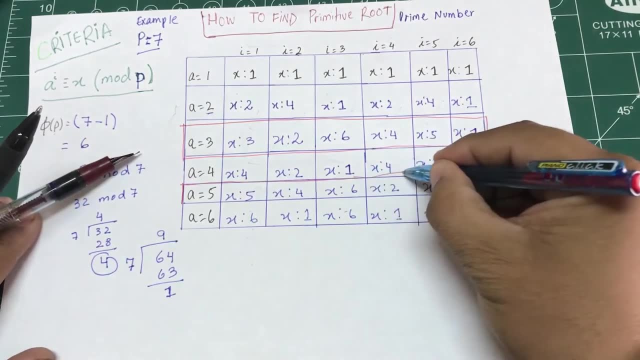 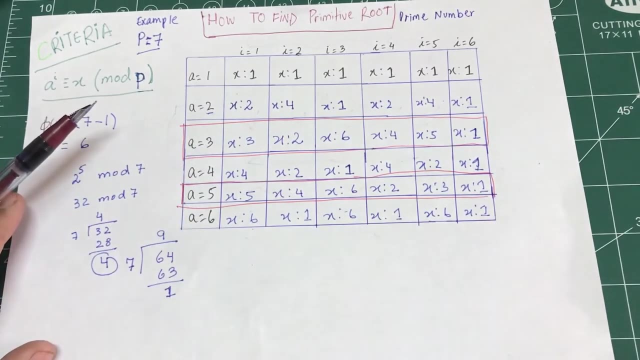 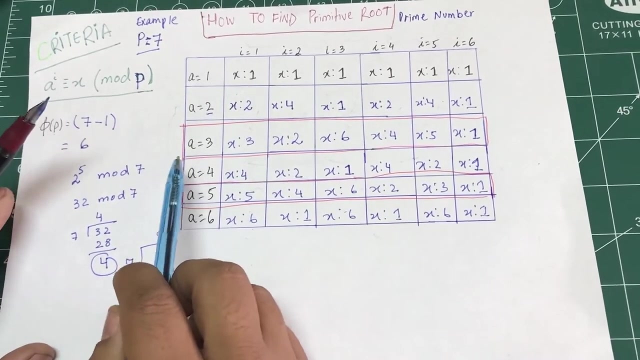 so one is three, and the other number that is generating this entire sequence is actually when a is equals to 5, if you were to look at this. so let's observe this: when a is equals, okay the thing. so what the primitive roots are, just to recap, is the number that is going to 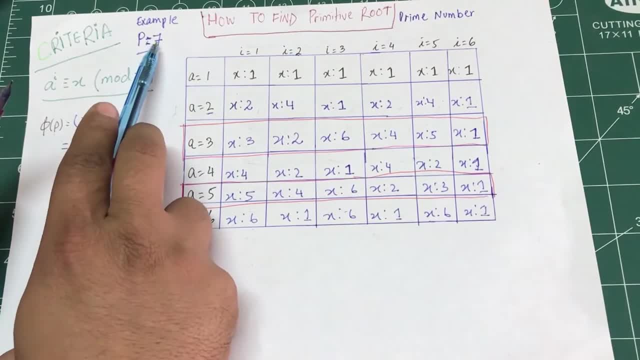 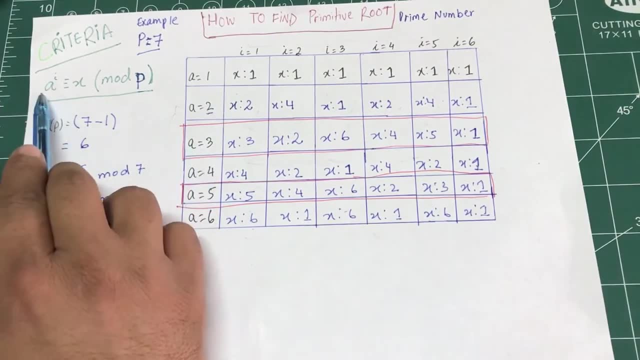 generate this entire sequence up till p minus 1. so since i have prime, which was 7, so 7 minus 1 is 6. so let's look at a. a is equals to 3. when a is equals to 3, is actually generating this entire. 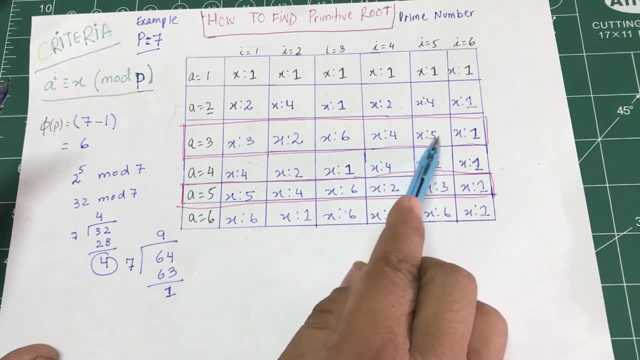 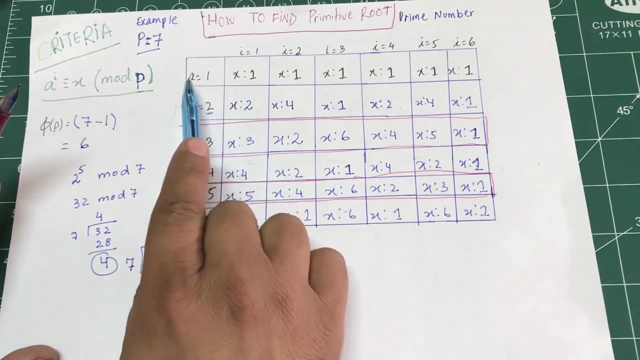 sequence. look at it: 3, 2, 6, 4, 5, 1. if i were to continue this further, while taking 3 and raising it to 7 after 1, whenever you see 1 after this, the same sequence will repeat itself. observe this. 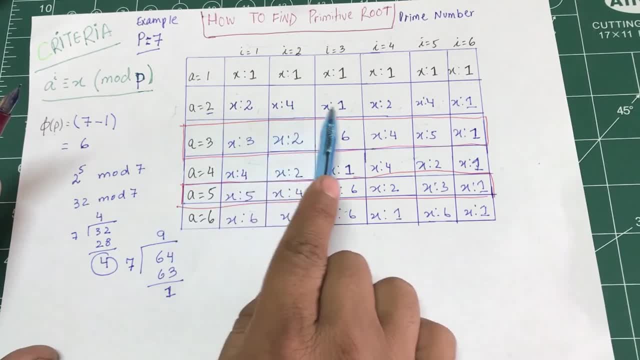 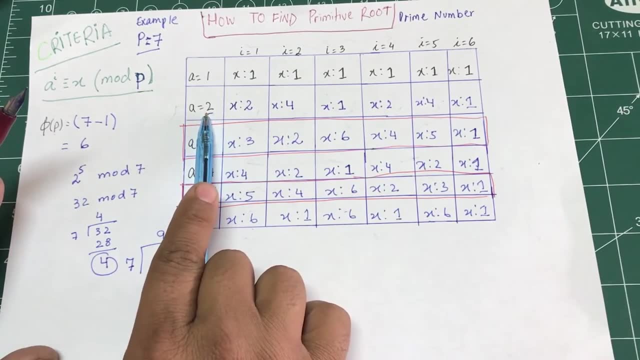 let's say: look at it: when a is equals to 2, we have 2, 4, 1. as soon as you hit 1, it start regenerating this. so, however, i take this a to be 2 and let's raise it to 7. 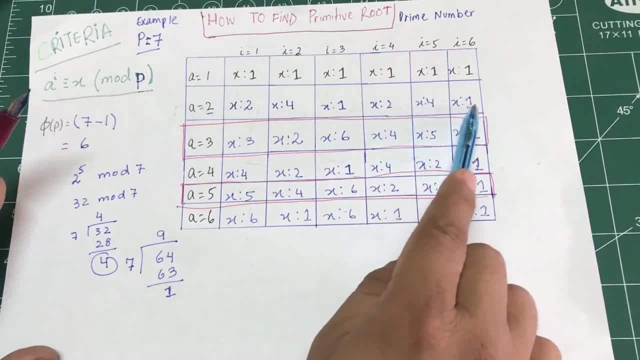 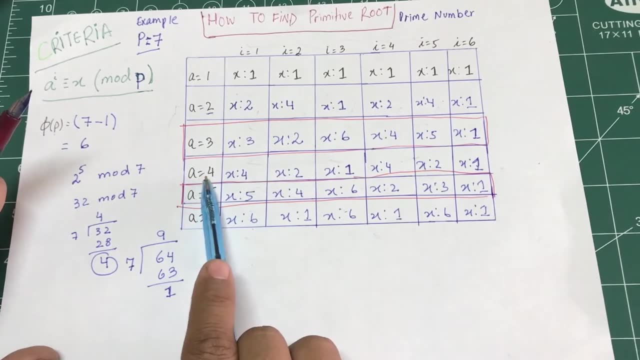 8, 8, 9, 10. it's just going to keep repeating this pattern: 2, 4, 1, 2, 4, 1. same thing when a is equals to 4. same thing when a is equals to 6. all right, so let's look at it: a is equals to 4. look at it. 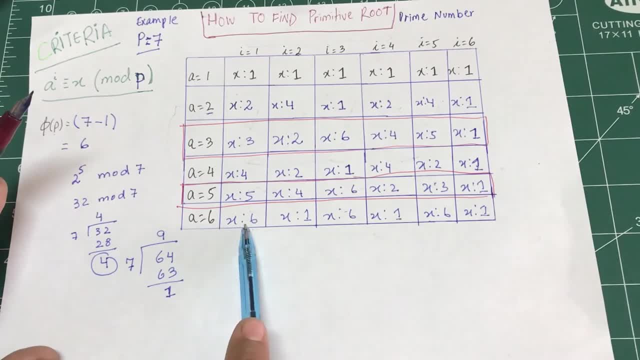 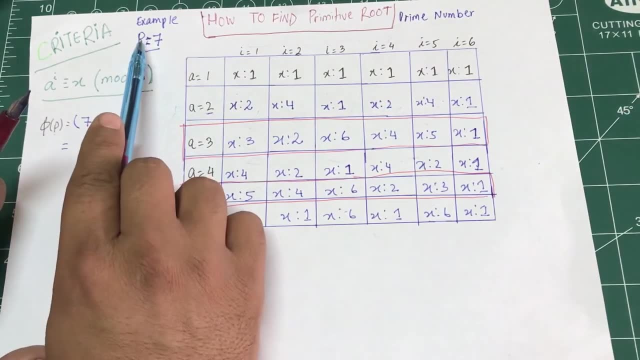 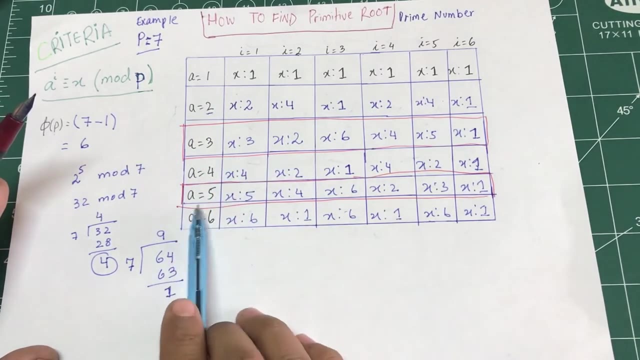 4, 2, 1 is repeating itself. 6, 6, 1, 6, 1, 6, 1. there's only two primitive roots of 7, of of of p is equals to 7. that is when a, those primitive roots are 3 and 5. look, 5 is also repeating the same. 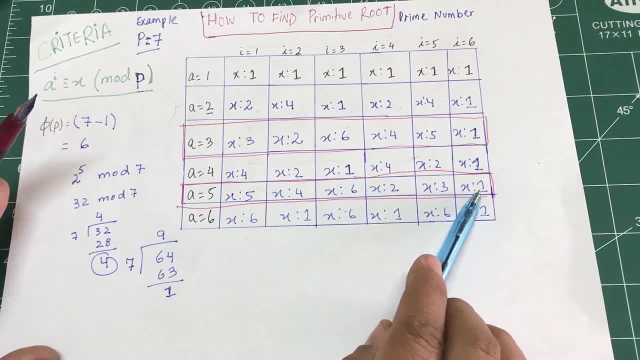 sequence: 5, 4, 6, 2, 3, 1. after this, if i were to raise 5, to raise to 7, i will get exactly the same element as 5, 4, 6, 2, 3, then 1. then it's going to keep continuing itself. so the primitive root.